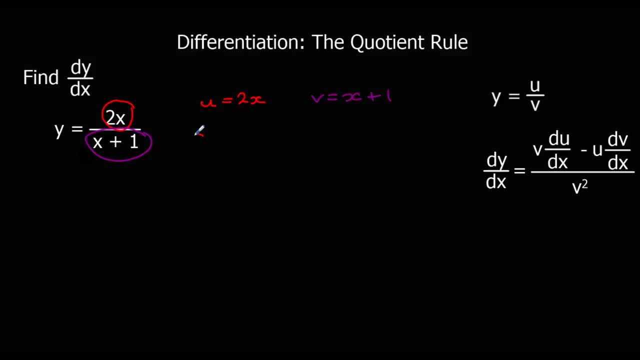 is x plus 1.. If we differentiate both of them, we've got dudx is 2 and dvdx is 1.. So then we just substitute these into the quotient rule and we find dydx. So dydx is v times dudx, v times dudx. so 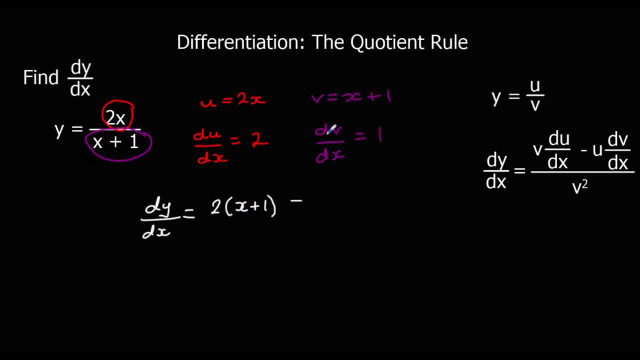 2 times x plus 1.. So dydx is dvdx, which is 2x over v squared, So x plus 1 squared. If we simplify by expanding the top line, we'll have: 2 times x is 2x, 2 times 1 is 2, and minus 2x We're going. 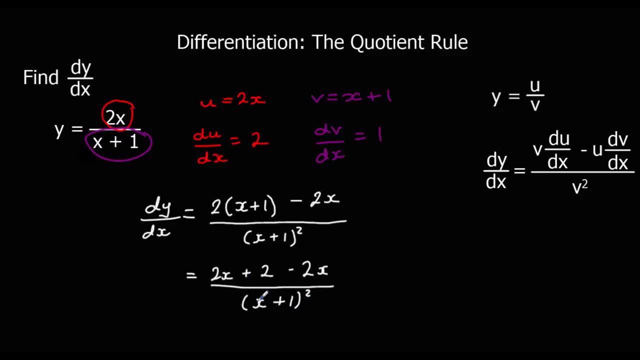 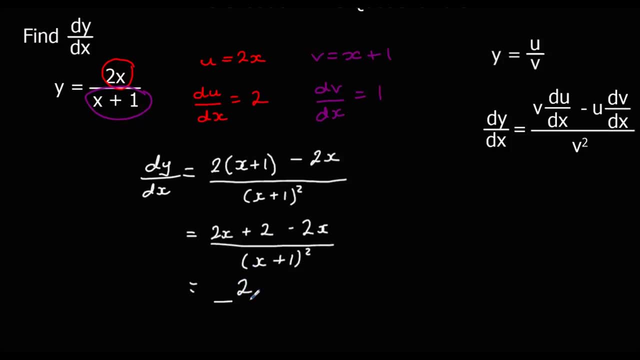 to leave the bottom as it is And we've got 2x minus 2x on the top. So 2x take away, 2x is nothing. So we're left with 2 over x plus 1 squared And there's dydx. 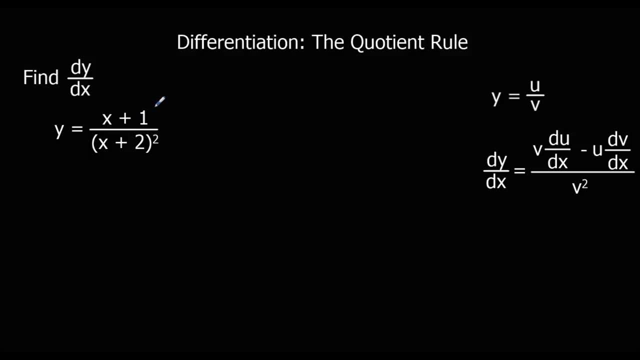 Okay, let's look at another example. So we've got a function on top. We'll call that u. So we'll say: u equals x plus 1 divided by the function on the bottom, And we'll call that v, So v equals x plus 2 squared. 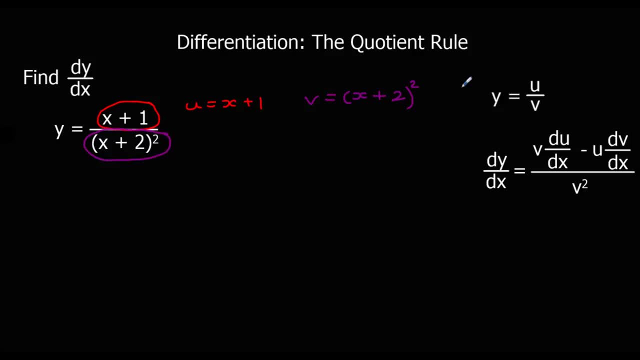 We're going to get a choice of which way round u and v go. for the quotient rule, u is always on top and v is always on the bottom, So we're going to differentiate both of them. dudx is 1. And dvdx using the chain rule. 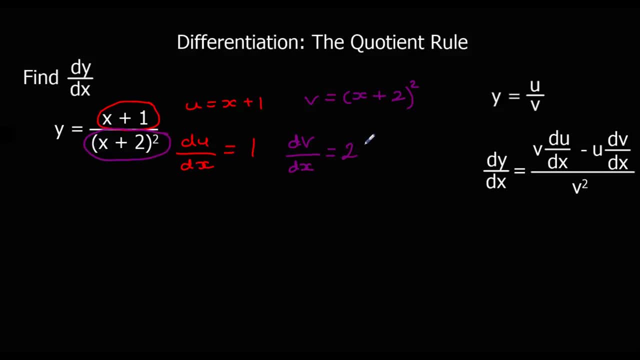 so we multiply or differentiate around the bracket to the power of 1, times by the bracket differentiated, which is 2. Which is just 1.. So we're going to leave it as 2 times x plus 2.. Then we just substitute in to our formula: So v times dudx, x plus 2 squared minus u. 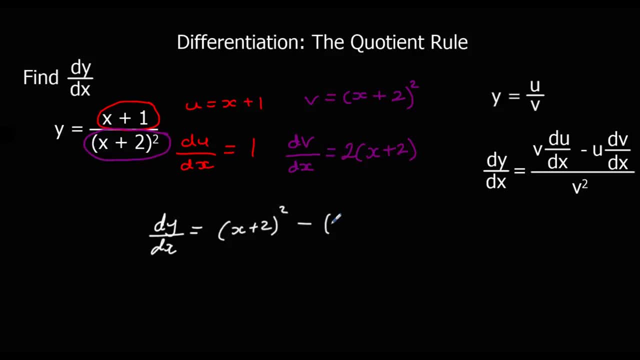 times dvdx. So we'll have 2 times x plus 2 times x plus 1.. Okay, All over v squared. So x plus 2 times x plus x plus 2. squared times x plus 2 squared is x plus 2 to the power of 4.. 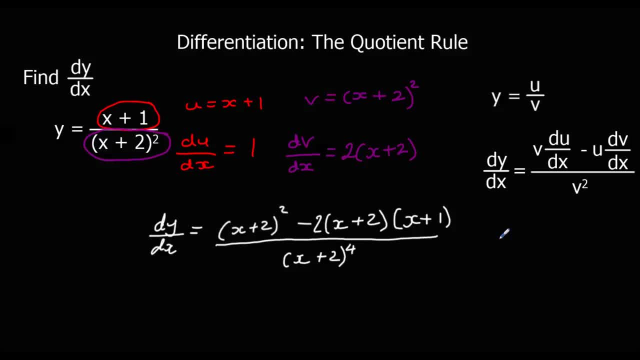 We could simplify the top line by expanding it and collecting like terms, but I'm going to leave it as it is Okay. Here's another example. Pause the video, Give this one a go. Okay, So we're going to say u is 2x plus 1. And v is 3x plus 2.. 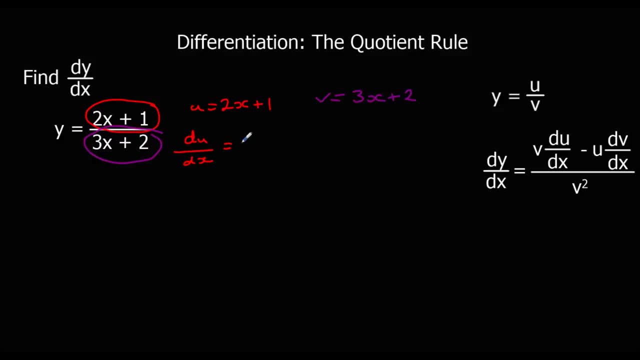 So that means dudx is going to be 2. And dvdx will be 3. So we're just going to substitute in to the formula now. So dydx, x plus 2 squared minus u times, x plus 2 squared minus u times. 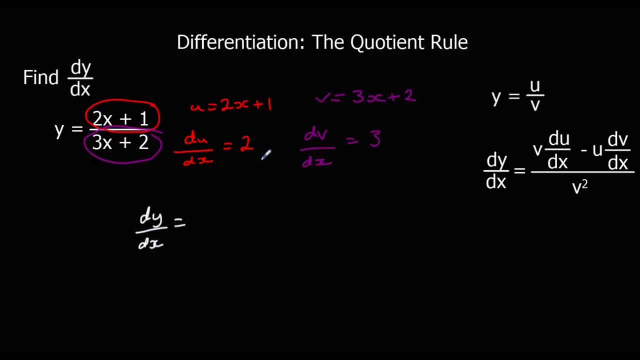 2 squared, So dydx is v times dudx. so 2 times 3x plus 2, minus u times dvdx, so 3 times 2x plus 1, over v squared, so 3x plus 2 squared. 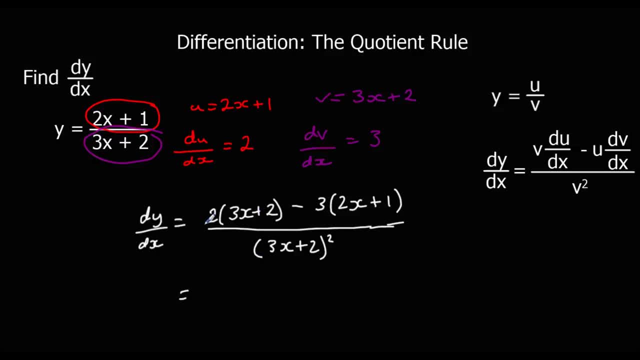 I'm going to simplify this one, So I'm going to expand the top line. So 3x plus 2 squared minus u times dvdx. so 3 times 2x plus 1, over v squared, so 3x. 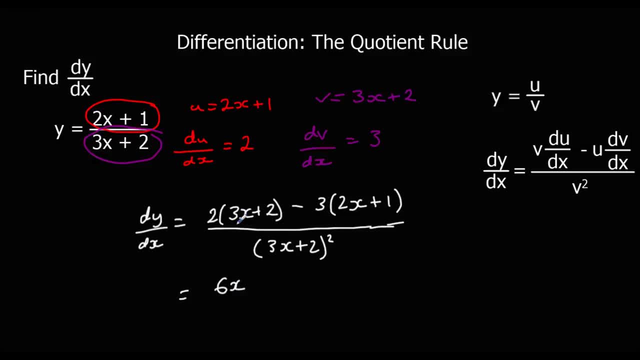 plus 2, squared 2 times 3x is 6x 2, twos of 4.. Minus 3 times 2x, So negative 3 times 2x is negative, 6x Negative. 3 times positive: 1 is negative 3.. 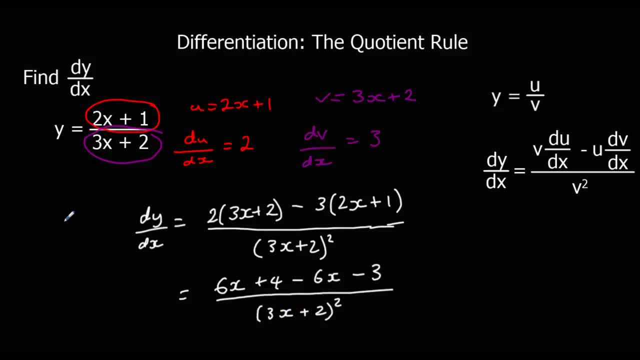 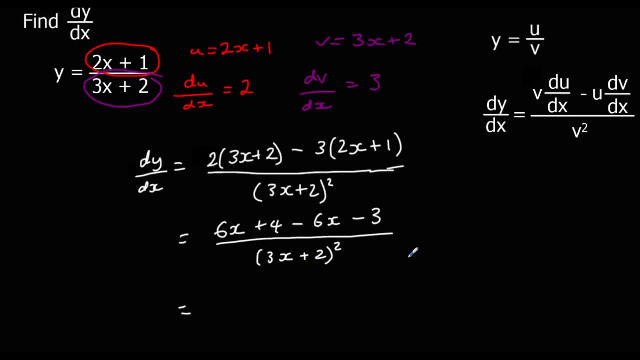 And I'm going to leave the bottom, as it is 3x plus 2 all squared, And then collecting the like terms from the top. So 6x take away 6x is nothing, 4 take away 3 is 1.. So we're left with 1 over 3x plus 2 squared.